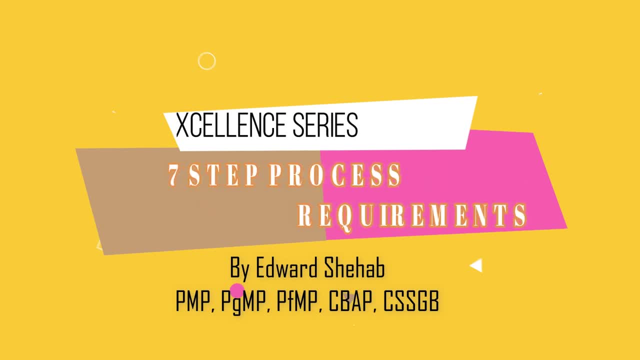 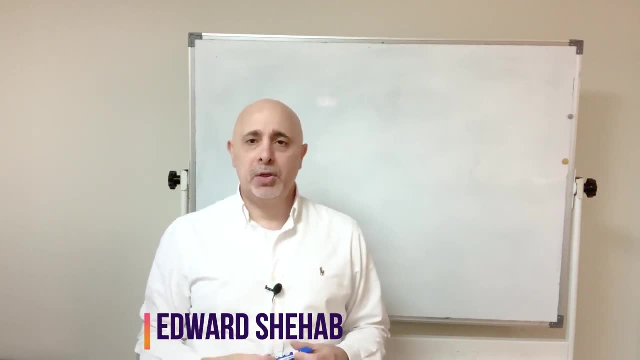 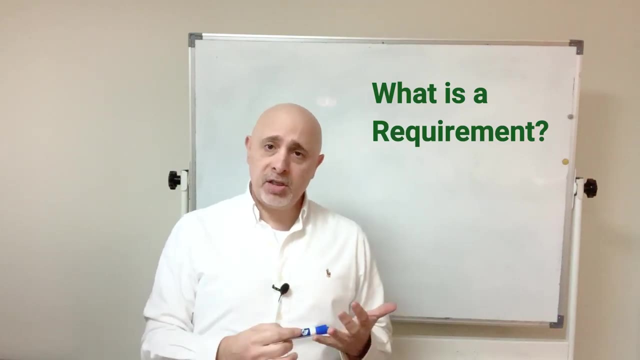 Hello, my name is Ed Shehab and I'm going to talk to you about a seven-step process for how you would go about collecting requirements for your project. First, let's talk about what a requirement is. A requirement is either a condition or a capability that is required from you by a stakeholder for a specific project. 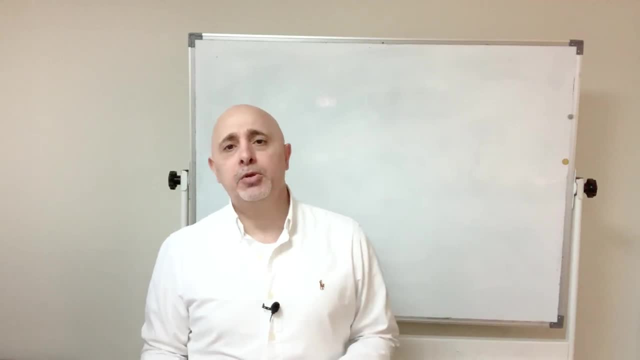 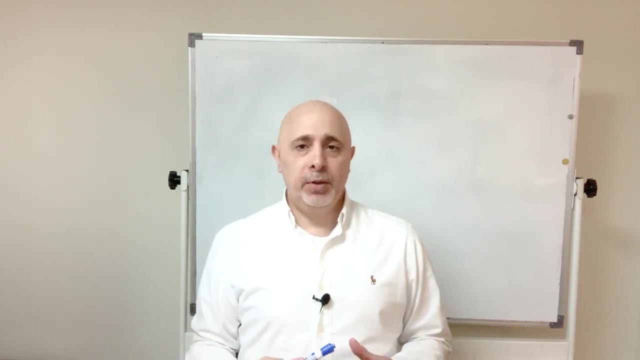 So when we talk about conditions, we might mean contractual terms, obligations, compliance requirements, timeframes or budgets or policies that you need to comply with. When we talk about capabilities, these could be features that your stakeholders need, So something like: it must be blue, or it must be eight feet high, or it must run at a certain speed. 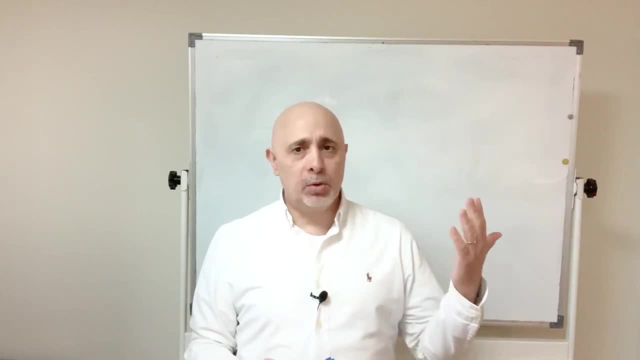 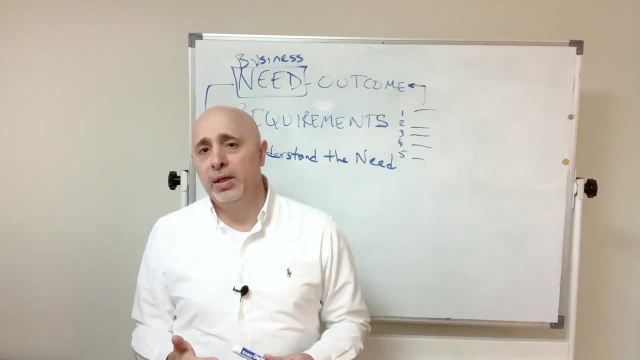 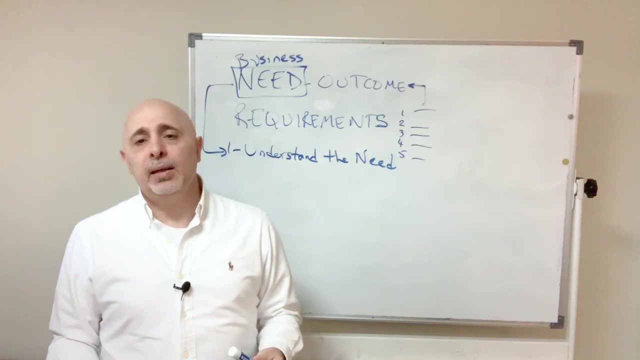 These are capabilities that your solution needs to have, So it's either going to be a condition or it's going to be a capability. The first step is understand the need. Your first goal is to first meet with the sponsor, or whoever is asking you for this, and understand what is their need. 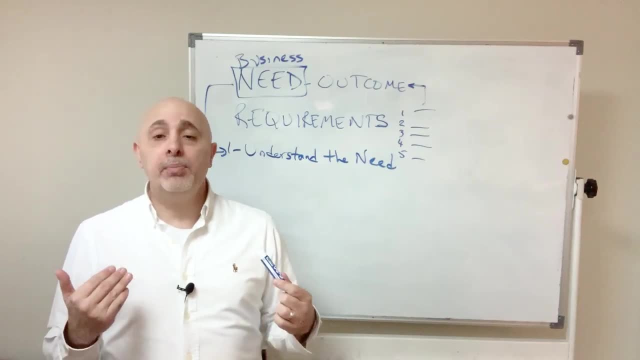 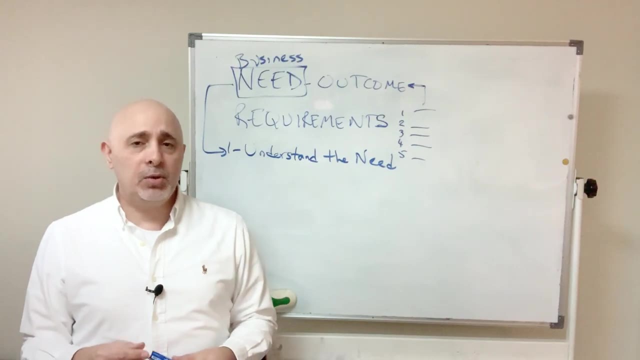 What is the outcome that they're looking for? Can you put some numbers against that outcome? Do you have all the specifics? Do you know how many people will be impacted by this? Do you know why they want this? What sorts of performance are they looking to get out of this? 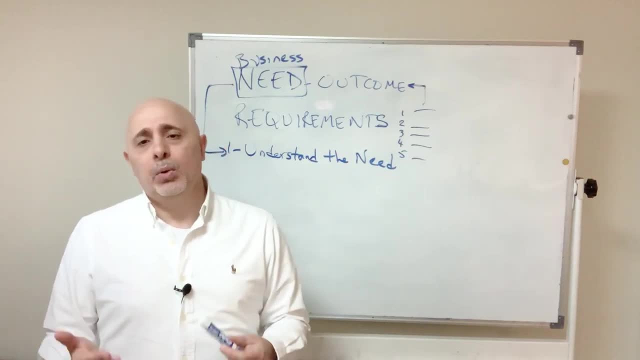 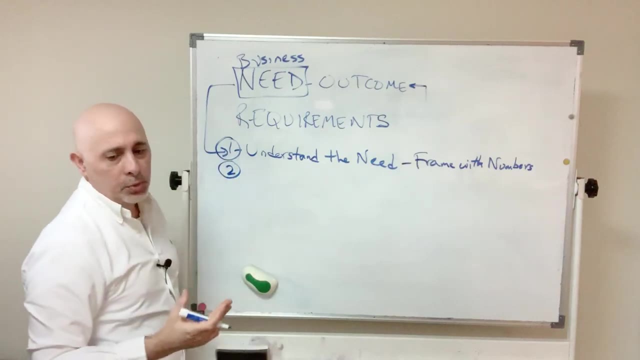 That kind of clarity Early on in the project will ensure that you're on the right track. So, assuming you are able to get a business need, then the next step that you want to do here is find out your limitations or your constraints. 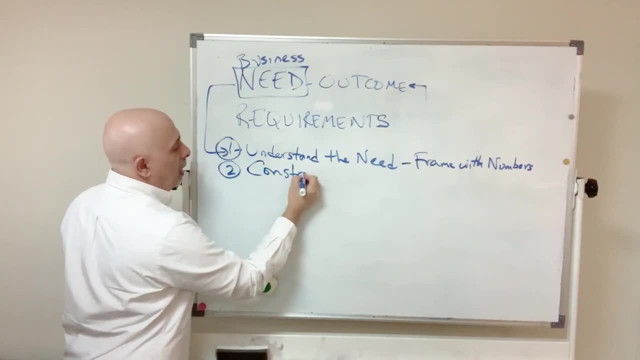 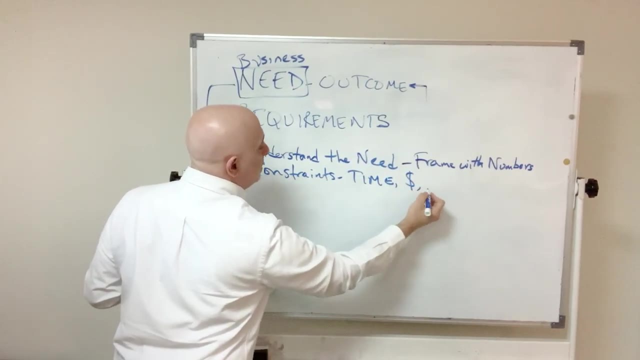 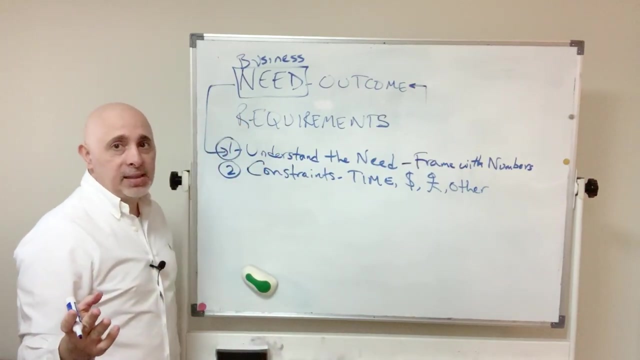 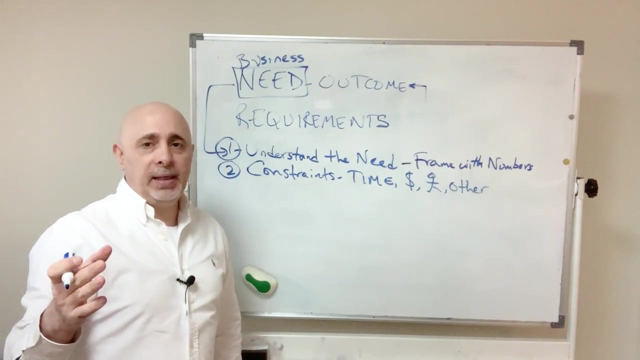 So ask yourself: what are my constraints? How much time do I have? So time is one of those, Money is another one of these resources And there could be some other constraints, Like rules and policies and regulations. So ask yourself what are the constraints that I have and put a plan- and you're going to put a plan- to deliver within that time frame or within that budget. 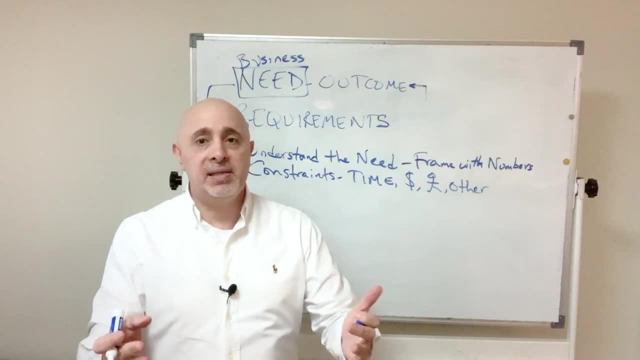 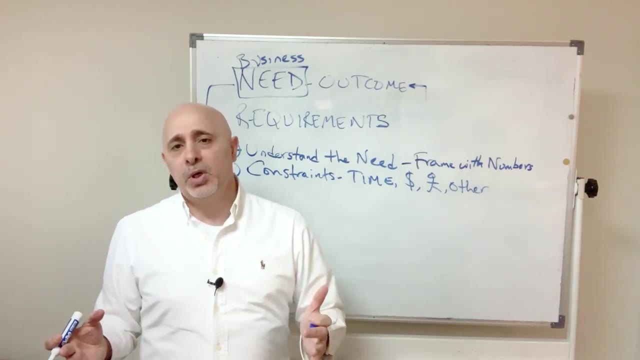 So, basically, if I have a critical need and I'm coming to you, you're the business analyst- and I'm asking you to get something done that we're looking to roll out in three months, then your business analysis process definitely can't take that long, can't take three months. 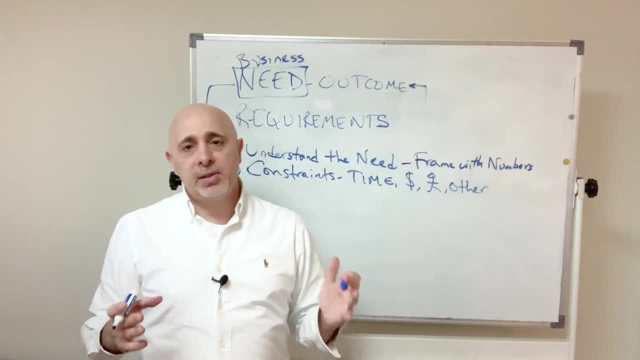 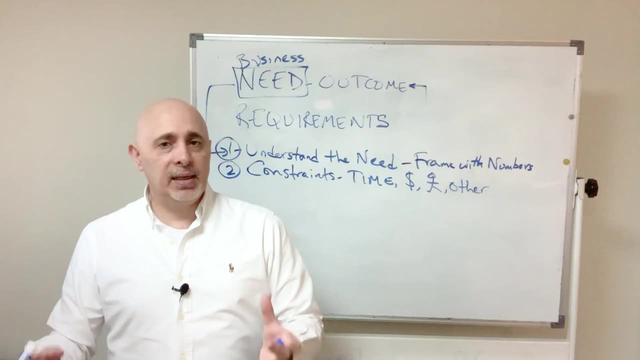 You probably want to take about a month, month and a half- Because you got to consider there's an implementation process, Somebody's got to go and code this and then they got to build the system and then they got to test it. So you have a very limited time frame to work with and that time frame you need to understand it. 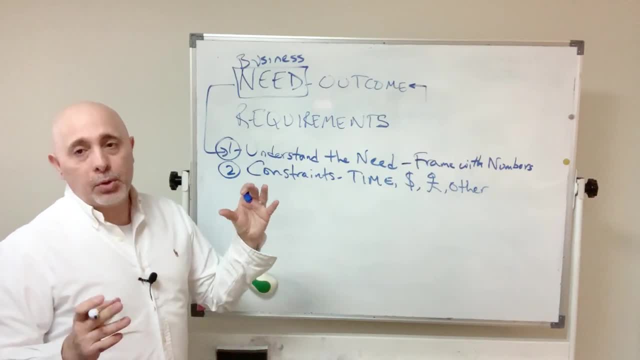 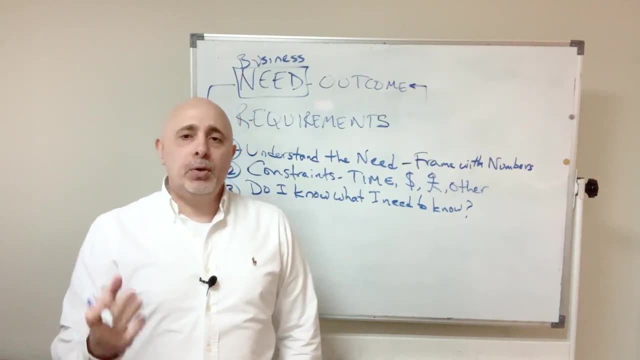 So, assuming you know what your constraints are, then you need to go to the third step. Do I know what I need to know? So what does this mean? Let's say you ask me to implement SharePoint across the organization, Or maybe you ask me to convert all of our printing into some centralized printing solution. 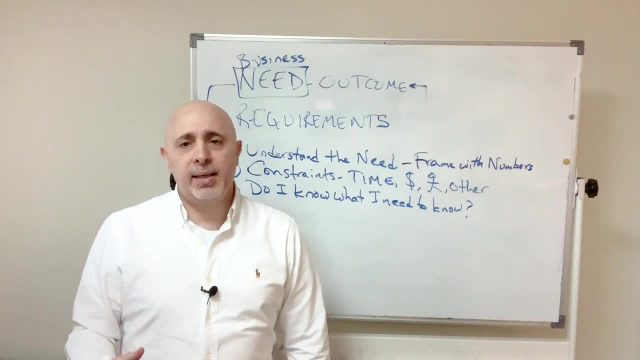 My question to myself would be: what does this take? Do I know the technology? Do I know how many people? Do I know the location? Do I know how much? Do I know what specific functionality you're looking for? Do you know? 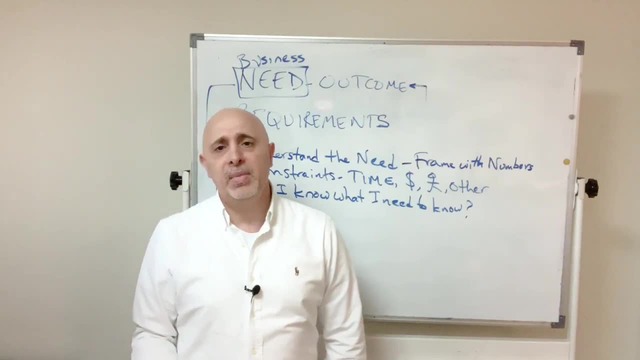 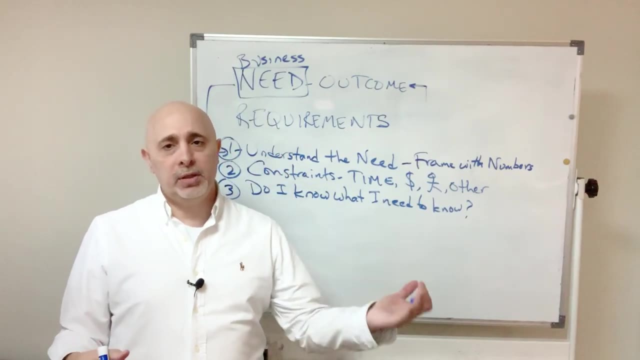 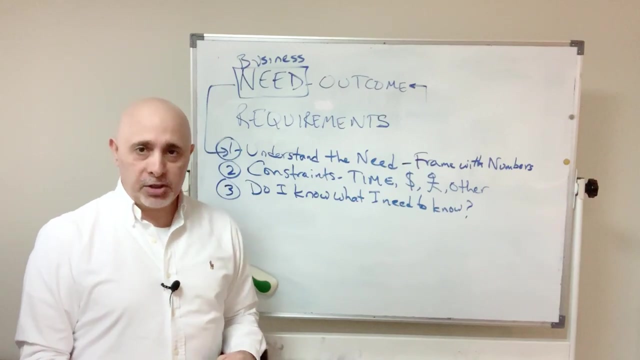 Do. I know the volume of work that is going to go through the system, So those questions that I have in mind are going to be answered by specific people or certain documentation. So in this third step, you want to know everything that is still missing for information. 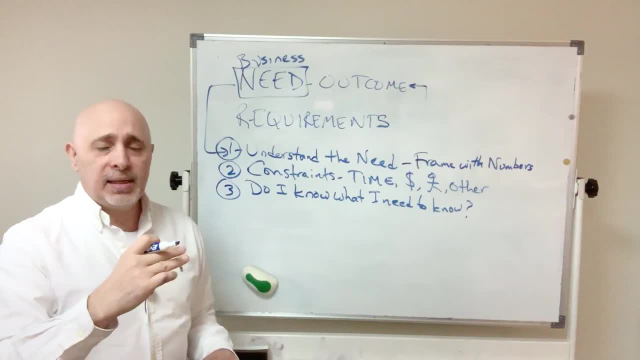 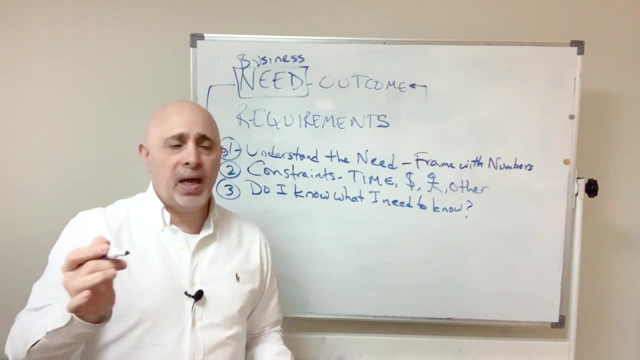 So now what you're going to do is create a list that says item number one that I need to know is how many people will use this solution. Item number two: how much are they willing to spend, Which was probably covered in step number two here in the constraints? 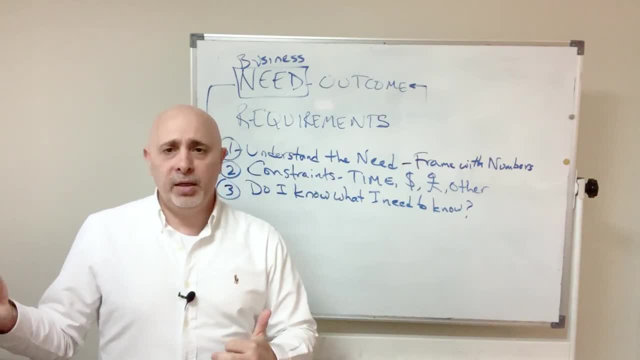 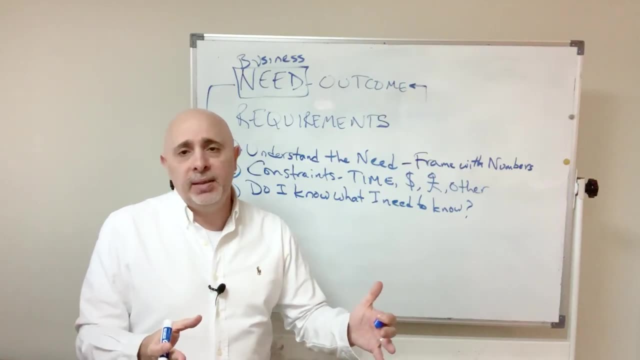 Item number three, for example, the location. Item number four: are there any rules that I need to follow? Item number five: what you know maybe what systems are in place right now that will need to be replaced by the new system? 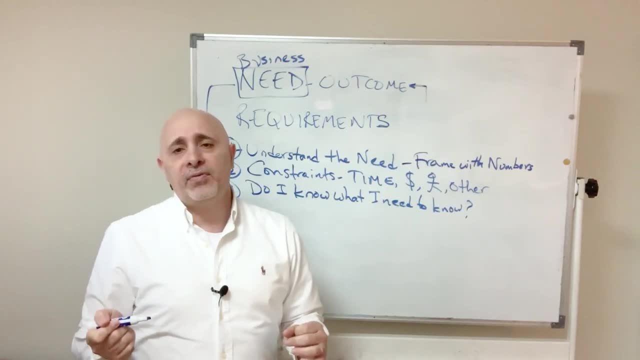 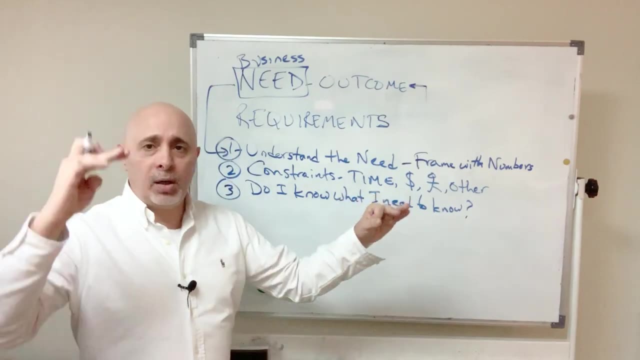 So you will need to figure out, you need to make a list of all the things that you need to figure out for this solution. So, assuming you figured out all the items that you need clarification on, then you go to step number four. 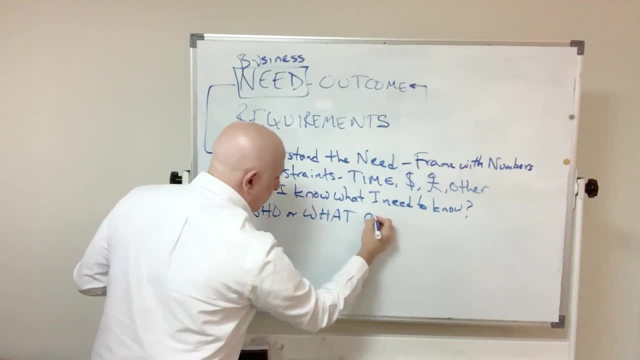 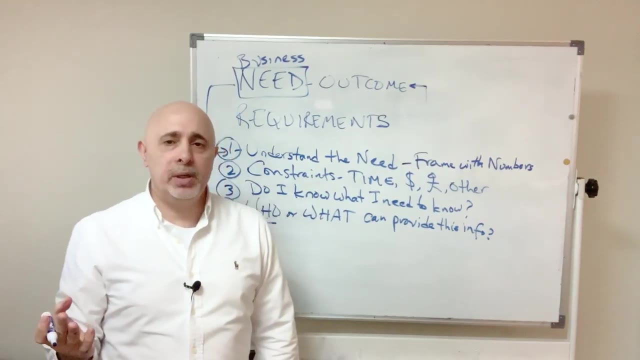 or what can provide me this information and the? who would be people. these would be your stakeholders in the organization. could be business managers, department heads, could be your colleagues, could be the admins who are going to be using the solution. so now you know, there are certain pieces of information that you 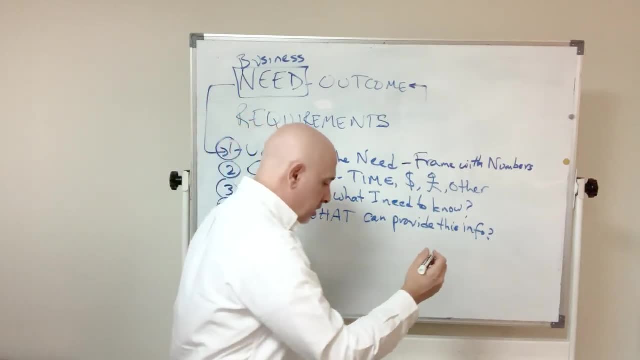 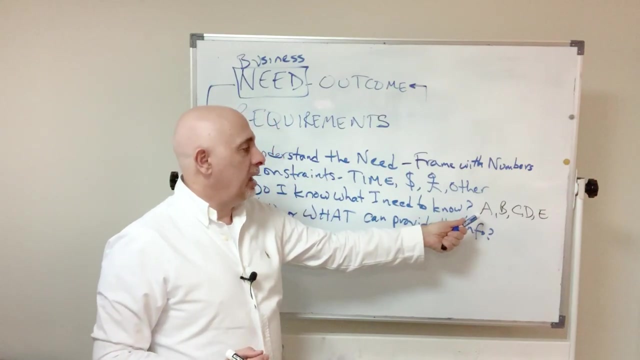 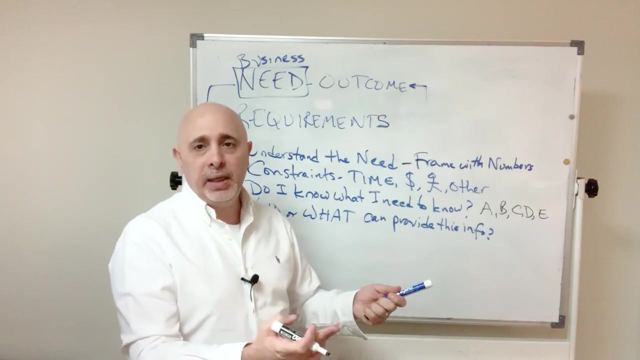 need to collect. let's say you needed to collect informations a, B, C, D and E. the question is: who provides me the information for a? who provides me the information for B? and if it's not who, then what? it is probably a document. it is probably something that is published on the internet, or maybe it's a supplier. 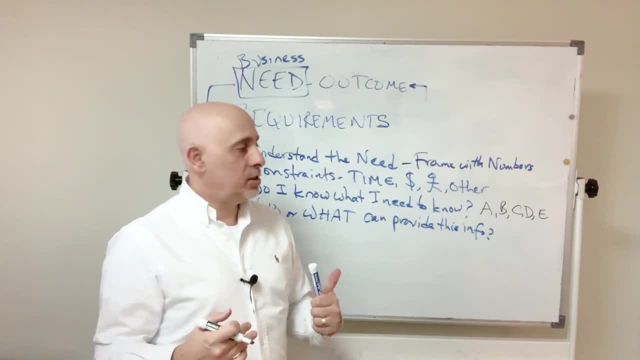 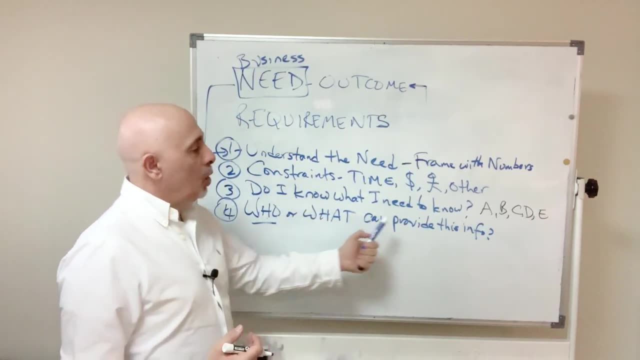 that you need to get in touch with who can provide you you such information. so here, what you want to do is you want to connect who, which is a P, which is a person, with the information that you need to collect. or, if it's not a who, it's probably going to be a document, a database or some form of 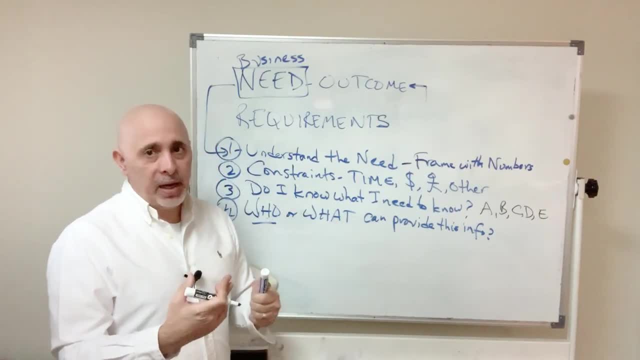 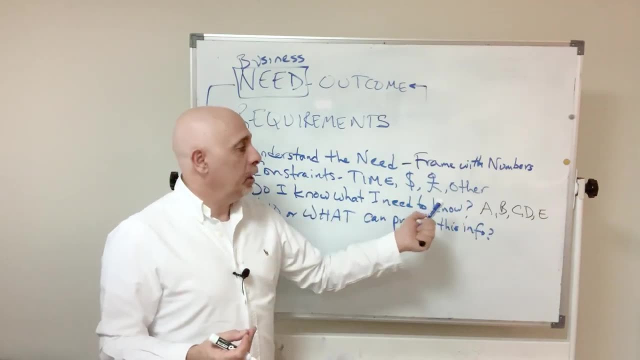 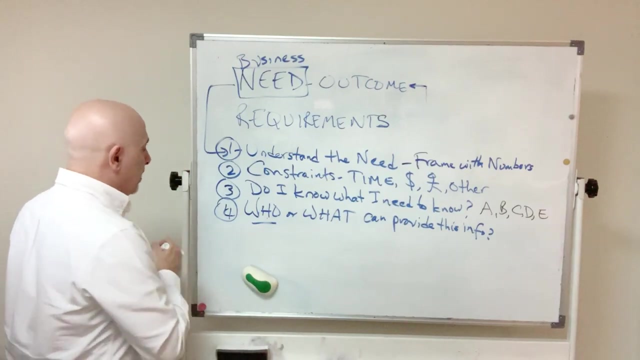 documented information, whether it's digital or in paper, but or it could be from a supplier, but what will provide you the information? so, between the who's and the what, you should be able to figure out the sources of where the information is going to come from. all right, so if you figured the 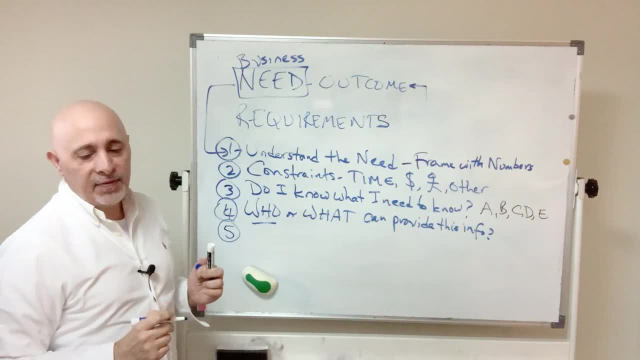 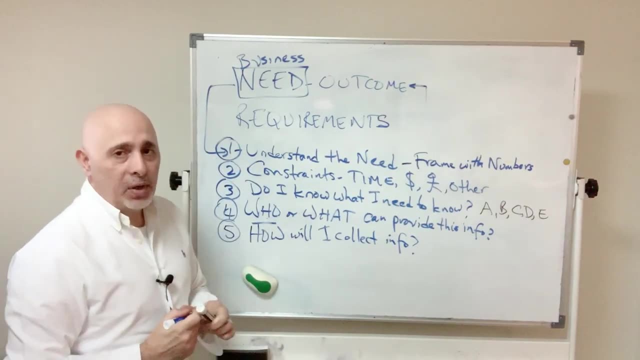 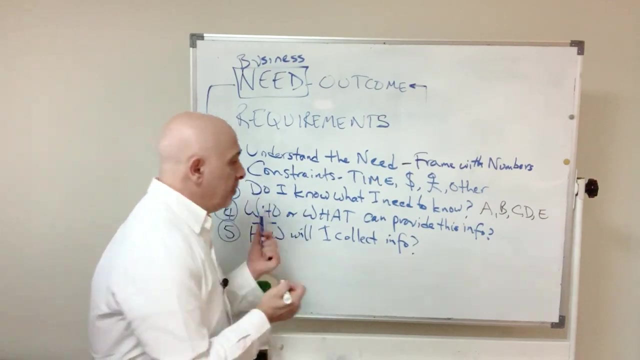 who and the what. then you go to the fifth step, and in the fifth step would be: how will I collect the information? now, the how, those are requirements, gathering techniques, and these techniques would vary depending on what it is that you need to collect. so step number five will be the techniques that 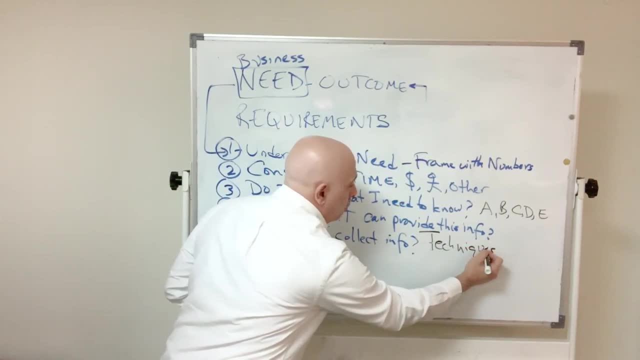 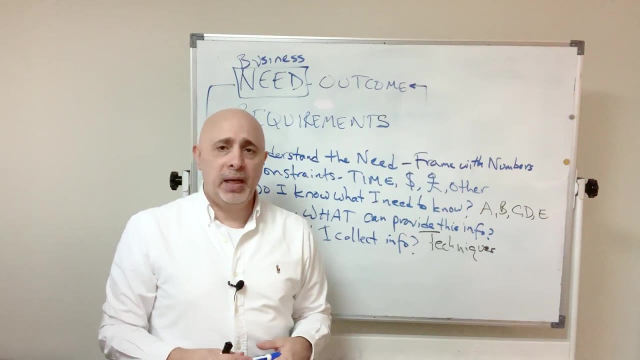 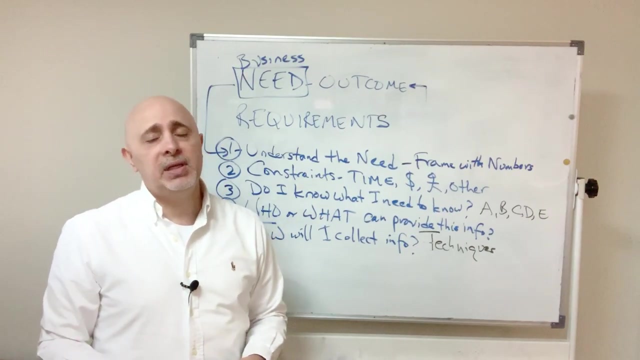 you will use in collecting requirements, interviews, workshops, focus groups, and you could also go to the what, which is, you know, document review and research, market research, benchmarking. you could reach out to suppliers, ask for manuals, review them. these are all the what's and the who's. you could also do a prototyping. you could do brainstorming sessions and 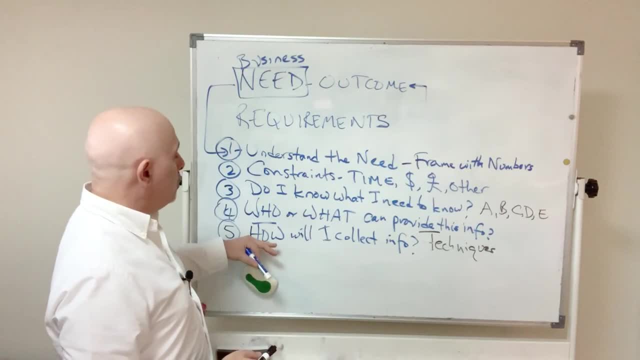 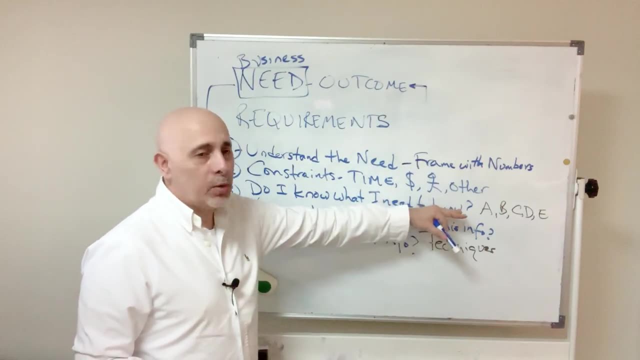 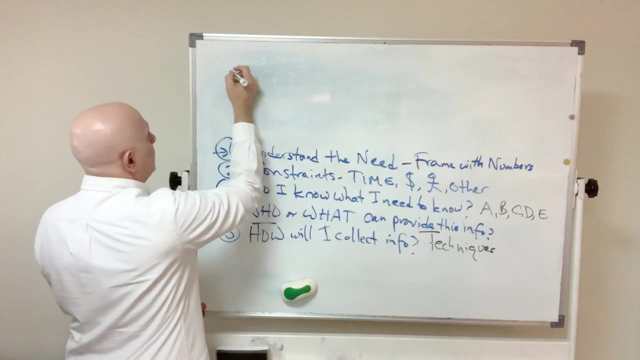 there's quite a few techniques. so what you need to do now is come up with a plan- not a plan, but a list- or identify, against every requirement, what technique you're going to use. and let's just say, I have a requirement. requirement one, for example, number of users. that will be. 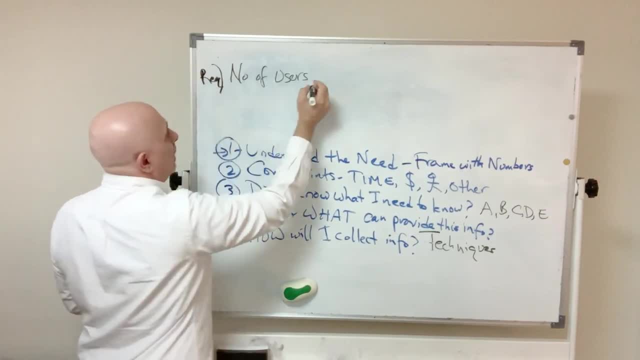 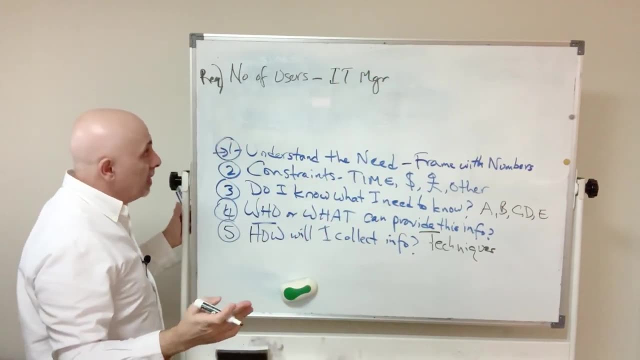 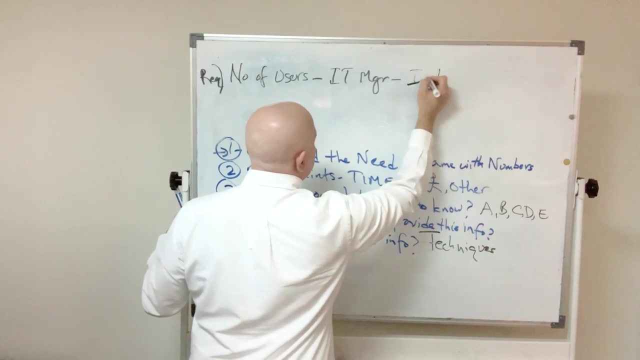 using this system. so that's my first requirement, right, and I figured IT manager is going to be the person that provides that information. then the next question, the next step, would be: how do I get this information from them? so now we have an interview, all right. so if I want to link them, that's your step. number three, that's your 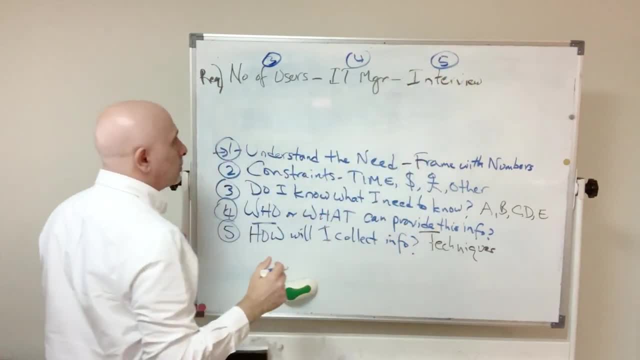 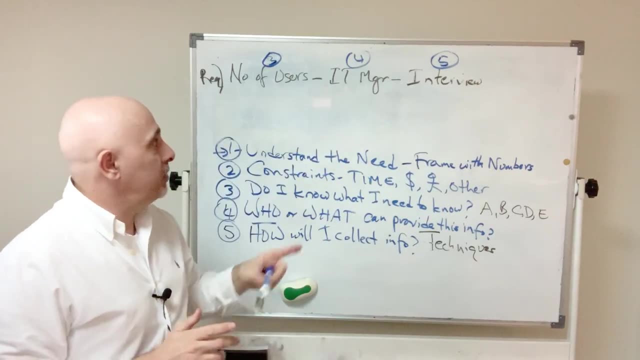 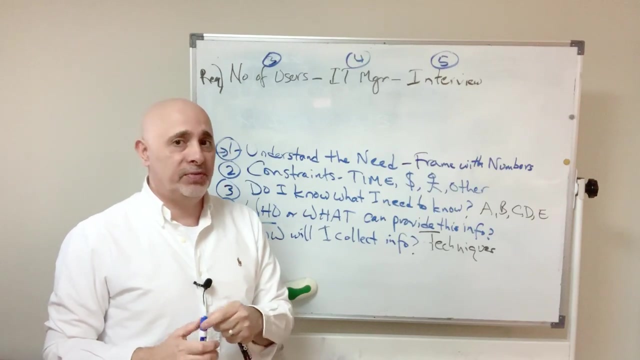 step number four. that's your step number five there all right now. this same IT manager is most likely going to be providing you more than this information. so number of users is one thing, but the same IT manager probably is going to provide you information on the technology behind it, or the interface. 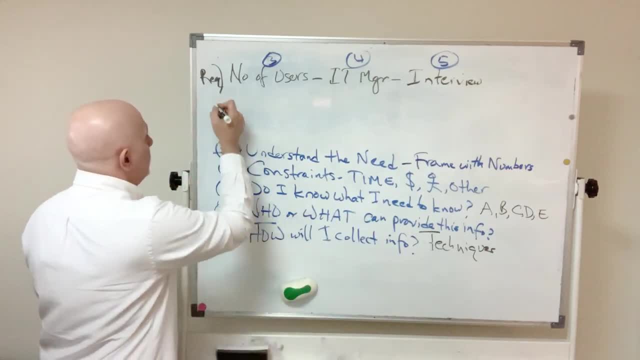 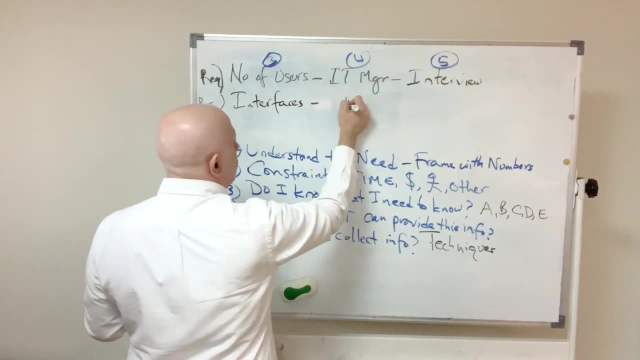 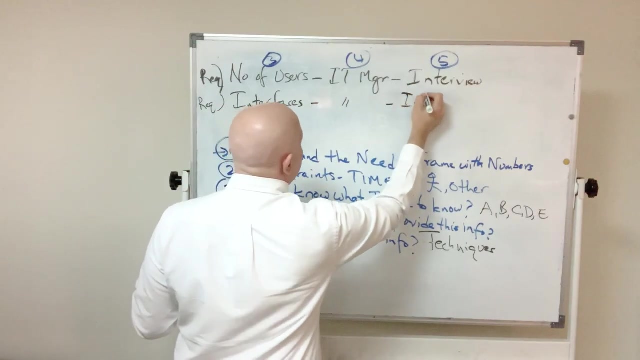 is required. so, let's say, your other requirement here is: so that's requirement number two: interfaces, and you have figured that it's also going to be the IT manager, and now the best way to get this information could be, and let's say, an interview, but it also could be a document review, where 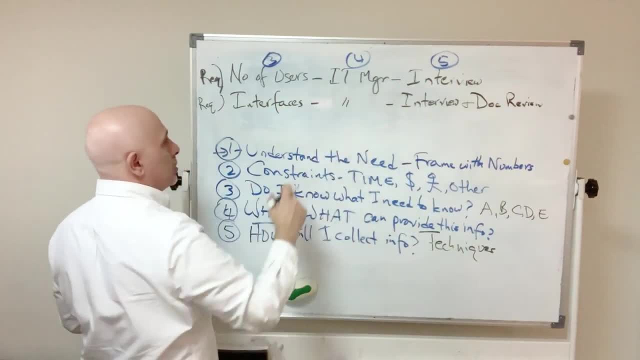 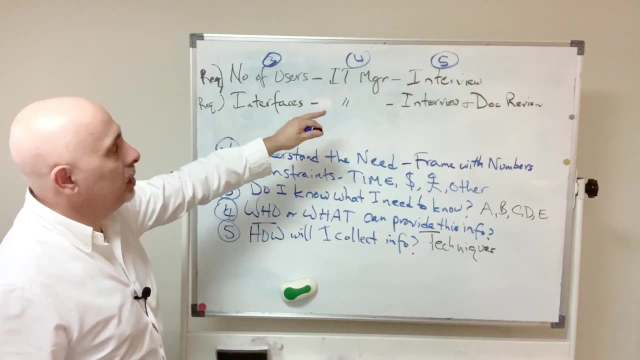 you have to review some document with this IT manager. so now you know that if you're going to be meeting with this IT manager, that you probably don't want it. you probably don't want to just talk about number of users. you probably want to discuss the 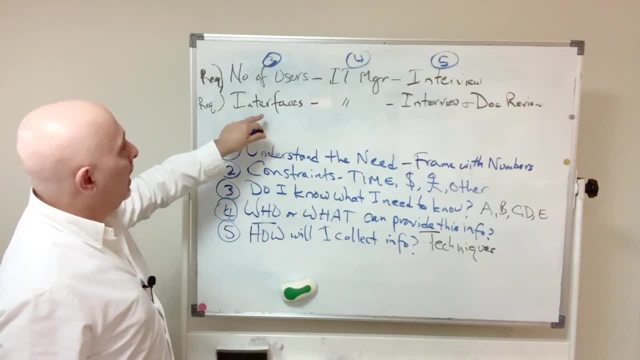 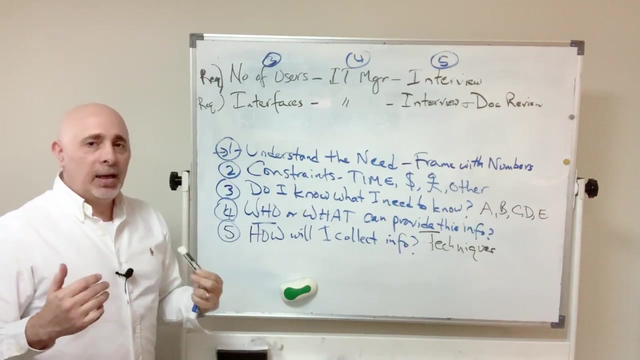 interfaces. so you would plan ahead and let this IT manager know that you're going to also review some documents in case they can get this ready for you. so here we see that some of these users needs the users and the time that you have to plan out in advance. who am I going to meet for which points? 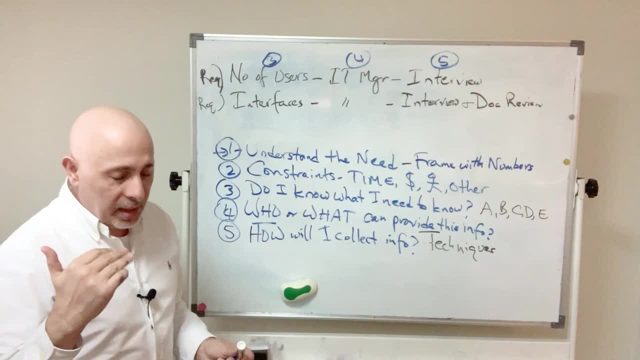 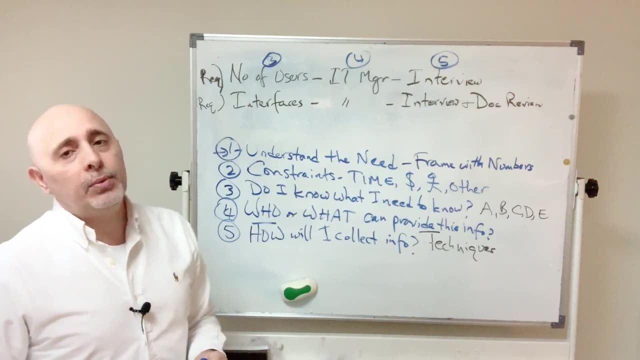 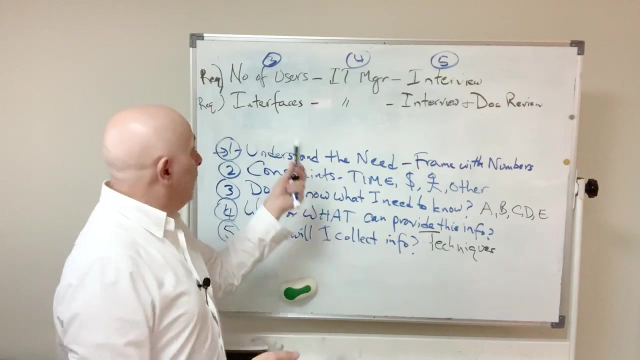 and you're trying to minimize the annoyances or the number of meetings that you're going to have. a lot of these users, and especially senior management, doesn't want to be troubled every single moment. you can't call them today and talk about number of users, call them tomorrow and talk about interfaces, and and then. 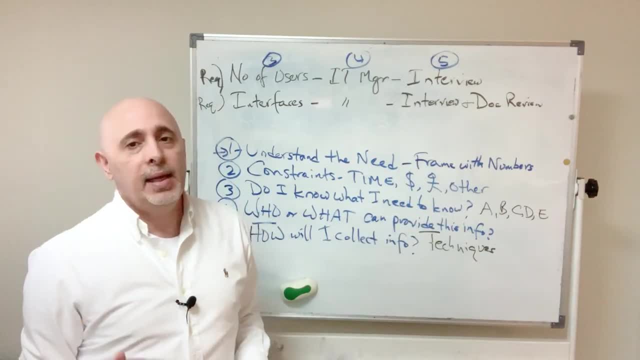 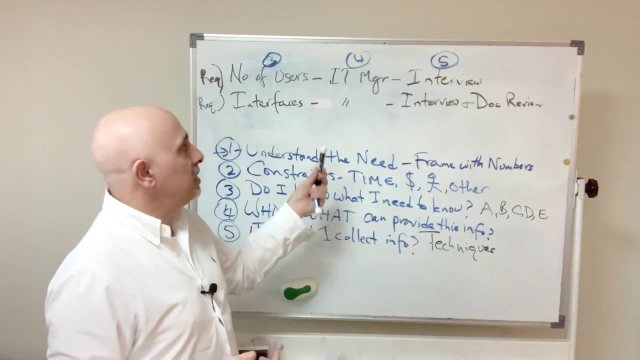 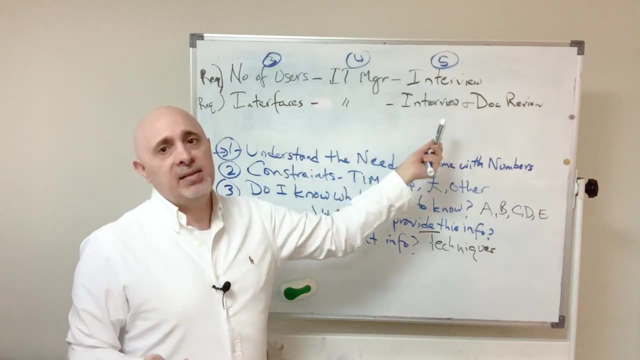 on the third day or one week later, call them and say, hey, I forgot this and you know, do you have a couple of minutes to discuss this? not everyone's going to be cool with that, so what you want to do is figure out, for every requirement, who or what is going to provide you this information. take a look at them and figure. 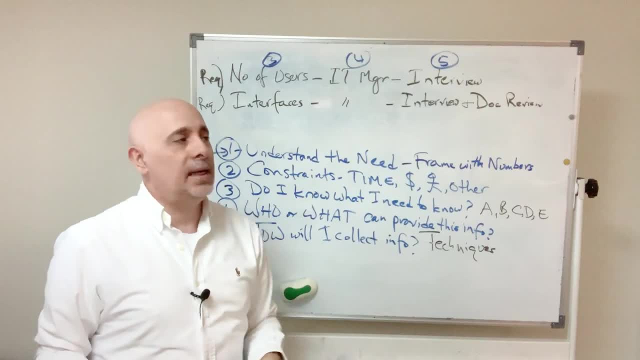 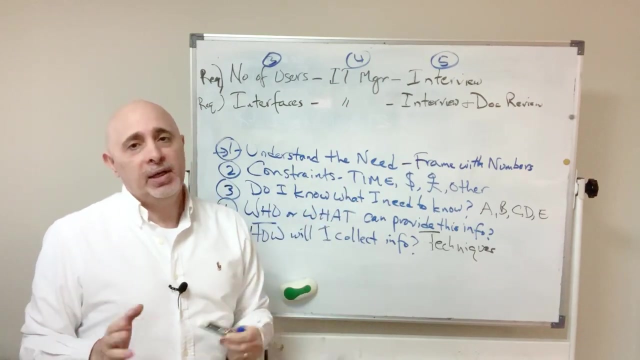 the best technique from you know, available techniques or well-known techniques that you would use to minimize the time frame for collecting the requirements. mind you, with regards to time frame, you also have to consider step number two constraints. you may have a limited time for you to get this done, and if you are really tight on time, then workshops might work much better than. 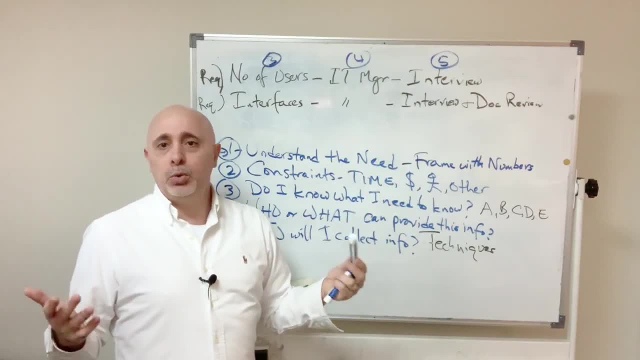 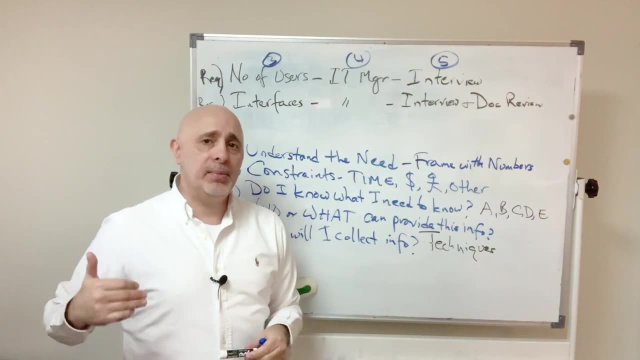 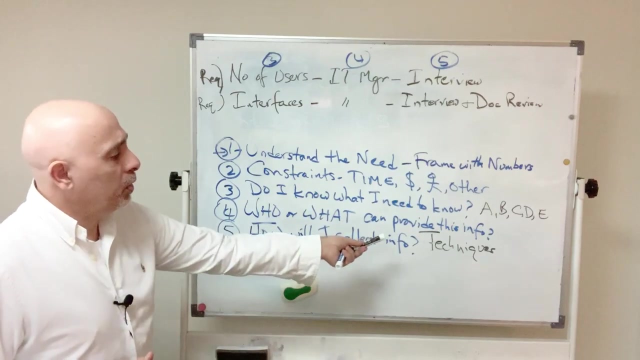 interviews, because you can just bring everybody there into a two or four hour workshop with some snacks and you can just sort things out. if you have a lot more time, then, yeah, interviews will probably be, you know, a good option for you to do. all right, so figure out how you're going to collect this information using 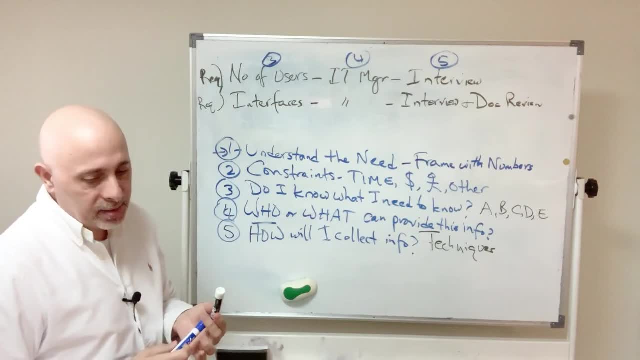 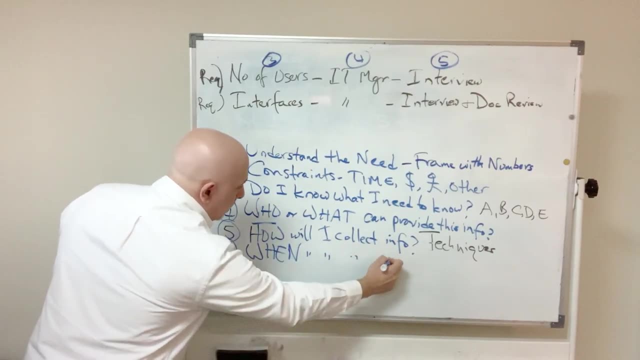 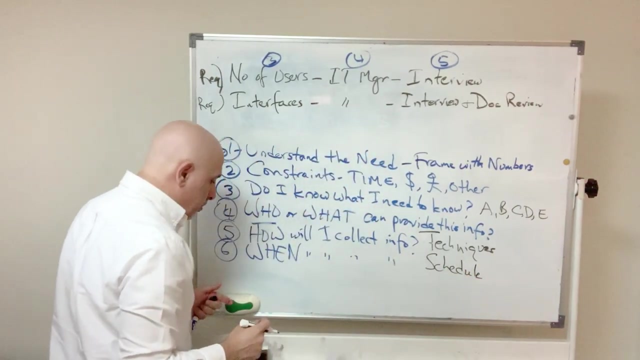 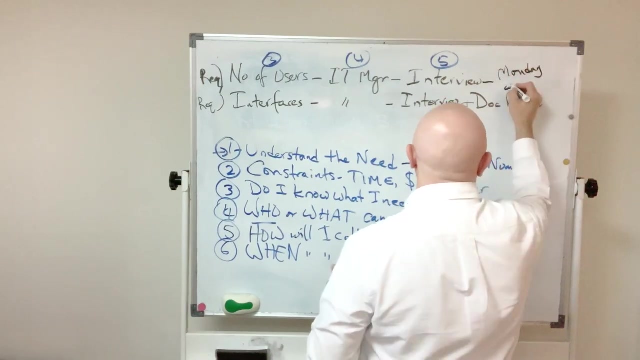 the techniques and then, once you figured all the techniques that you want to use now, go to step number six, which is when will I collect info? and that would be your schedule. so you're going to develop some sort of a schedule and that you can just put at the top here. so if I want to figure here that let's say I planned for Monday at 9 am. 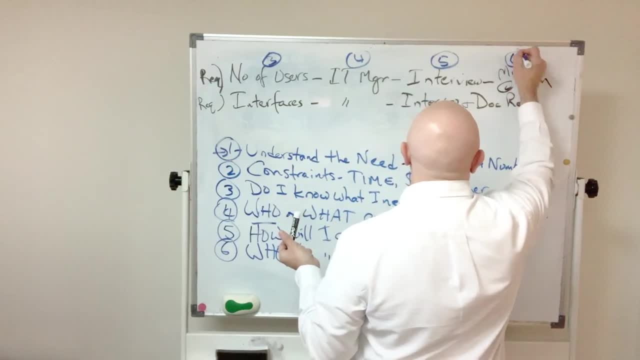 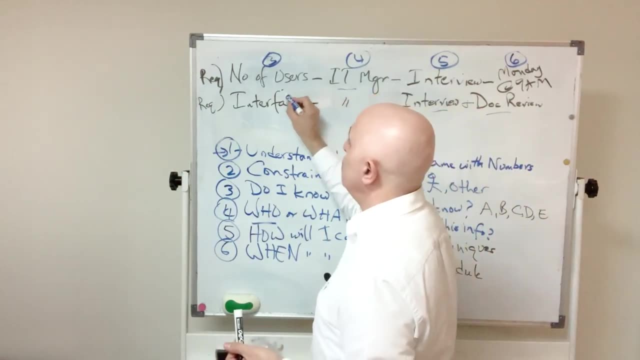 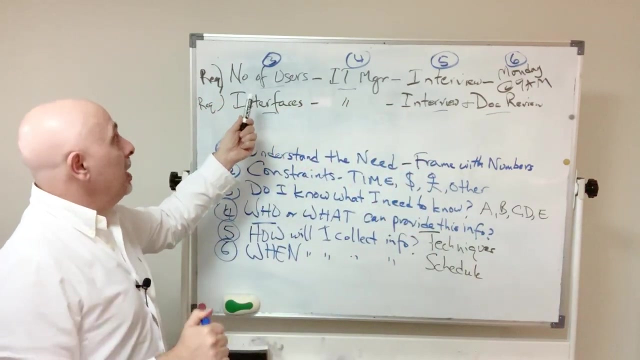 that's step number six for me. I figured Monday at 9 am I'm going to do an interview and review some documents with the IT manager to understand these key points. does that make sense? so here, step number three, number of number of users, is a requirement. and step number four: this is who's 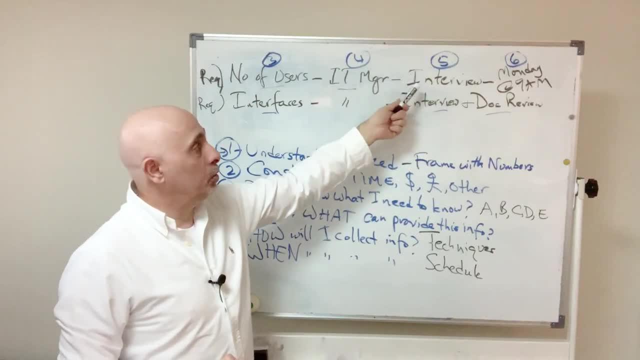 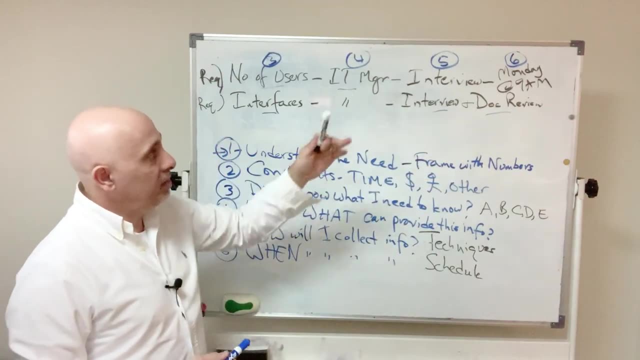 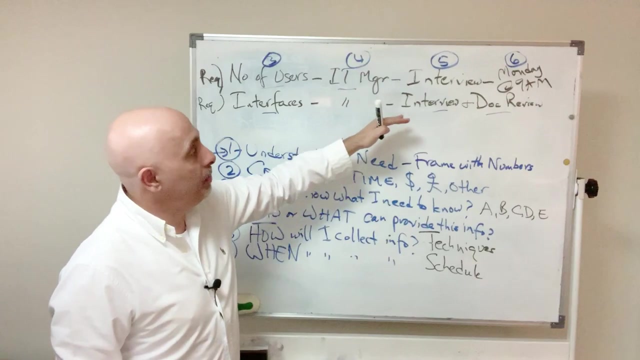 going to provide it. and step number five: this is how I'm going to get this information using that technique. step number six is when I'm going to get that information. so when you develop the schedule, as I previously discussed, you probably want to plan out, plan out the best and the best timing. 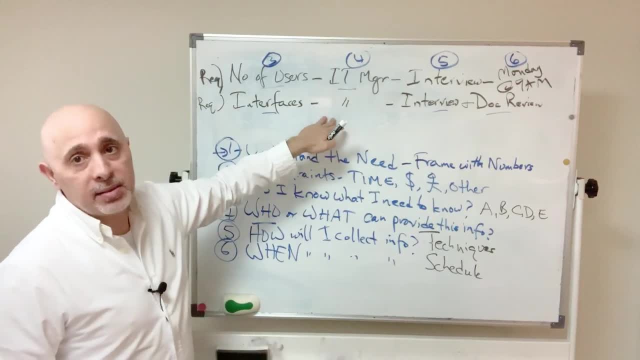 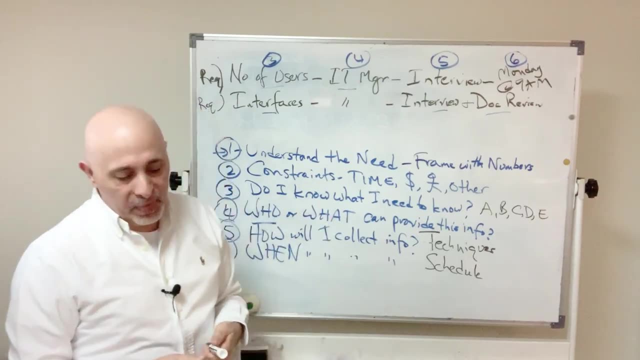 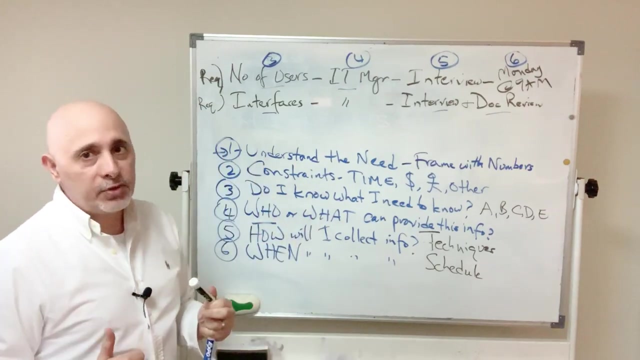 or duration or techniques that will minimize the number of interactions that you're going to have with these stakeholders, so that they don't get bothered by what you're doing. so now, let's say you've developed a schedule: Monday at 9 am, Tuesday at this time, Tuesday in the afternoon, I'll meet this guy or we will have this. 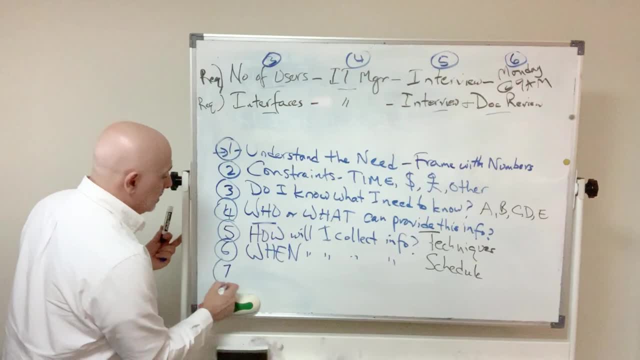 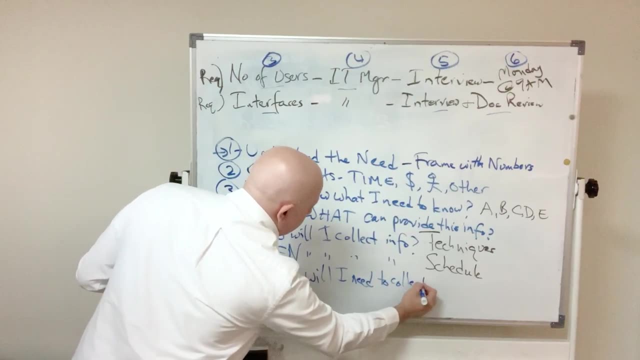 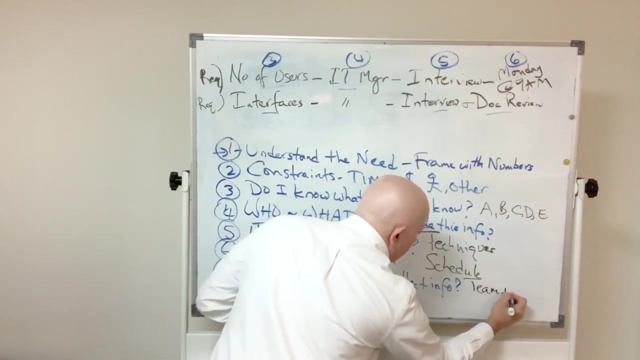 kind of a workshop. then the next step that you want to do is ask yourself: what will I need to collect info, and in this step what I mean is people or tools. so here I'm just going to write people or team and tools. so you have to ask: 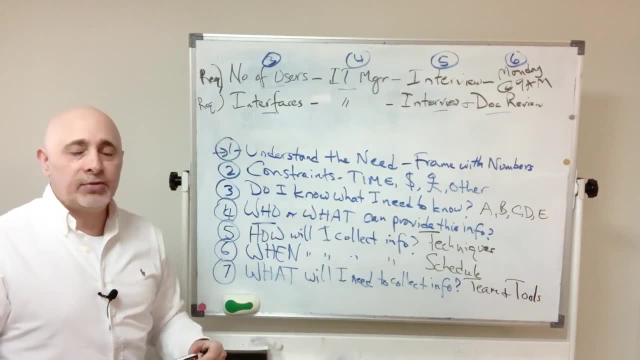 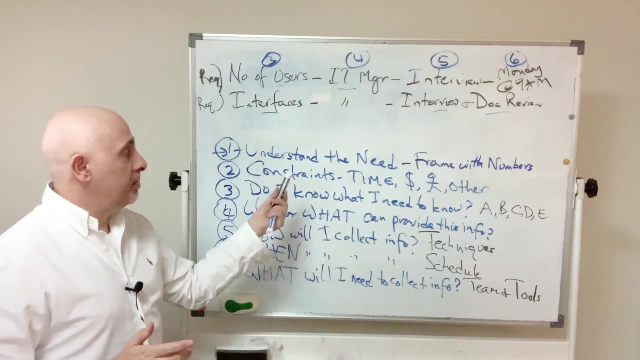 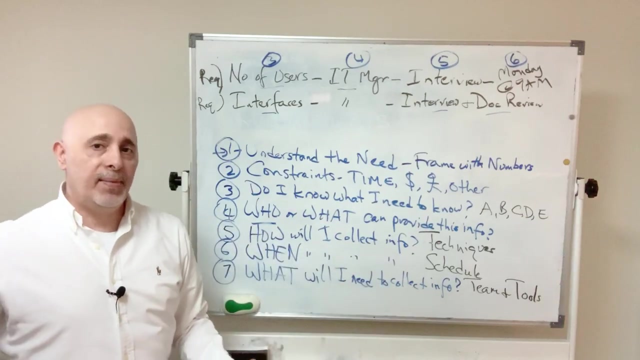 yourself? do I? is this something that I can do by myself? do I need a team? do I need someone to help me for the time frame for step number two, where I have limited time or limited money? what can I afford for people? would I be able to do this myself by looking at the schedule, if it looks? 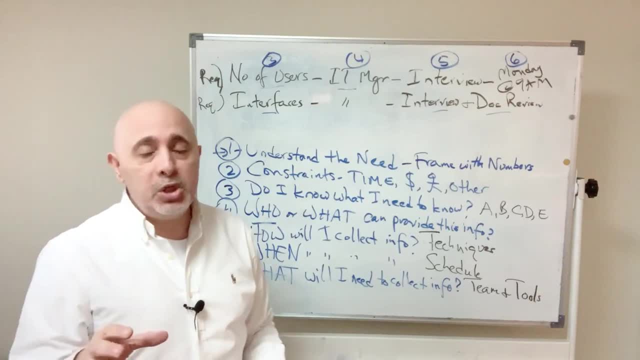 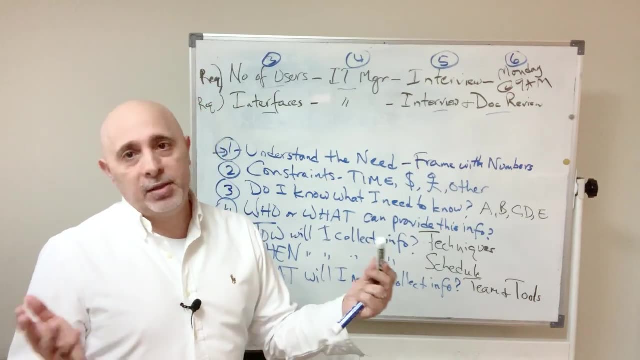 like you need three months to get something done and your management is pushing for something to be done in one month, then obviously you're going to need some help, and agreeing to do this by yourself would be just, you know, suicide. you're just trying to um, you know. 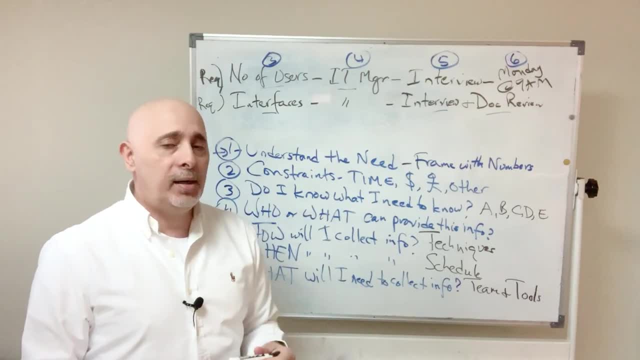 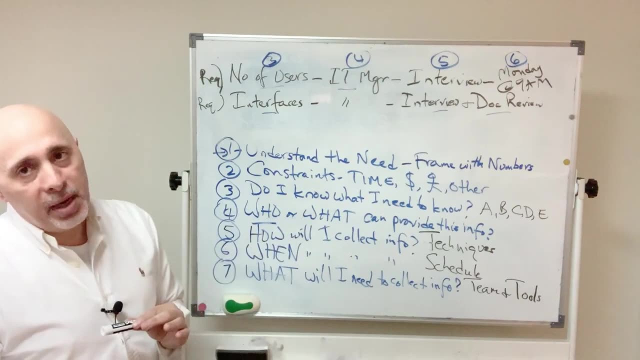 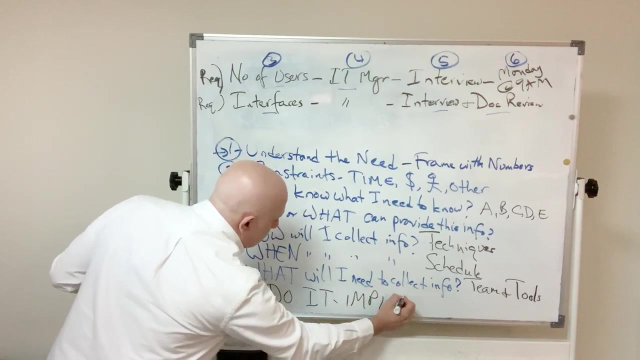 you're leading yourself to failure and you don't want to do this. you're trying hard and for that you know you need to ask for all the support now. if you're able to get these people, the team and the tools, you can go ahead and implement your plan. you can just go to implementation at this point. 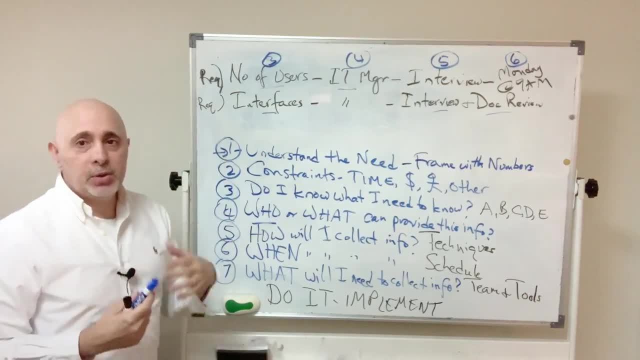 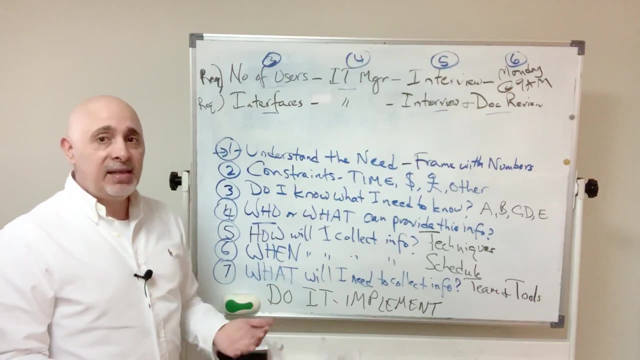 so, just to recap, you first get a need from your senior management. they ask you to find a solution, a brand new solution, or a replacement or an enhancement for something that you have in place. the first thing you want to do is meet with them, understand the need, try to frame that need with 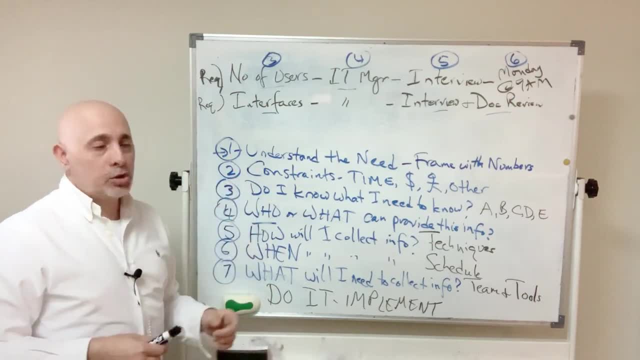 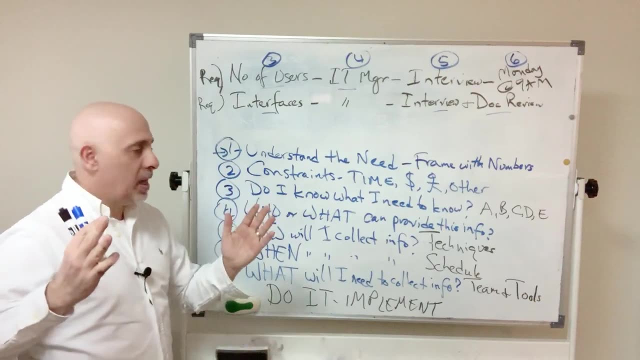 numbers, whether it's a problem or an opportunity. find out what the constraints are, which is step number two: time, money, people, resources, location. find out what it is that they've put for boundaries for you. and then, step number three, ask yourself: what do I need to know for me to get this done? and you: